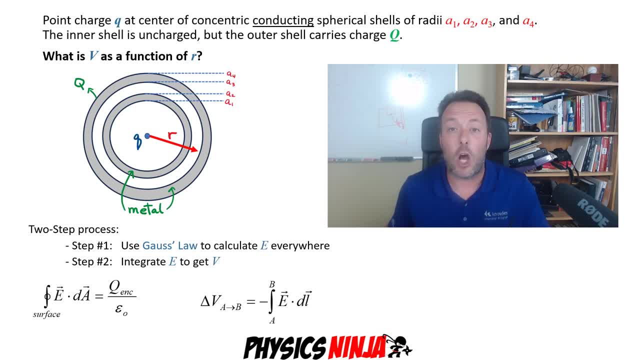 potential. There is nothing wrong with that technique, but it is hard, okay, It involves a lot of work. So, in addition to that, I'm also going to show you an easier way to do that, based on the result of one of my previous videos. And here's what the result of the previous video says: 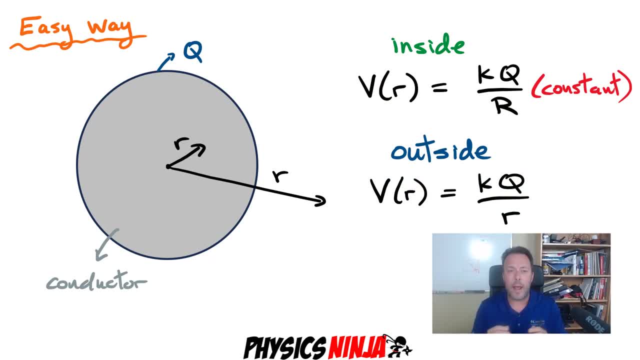 It says: this is what I consider the easy way. The easy way says that if I have a conductor, whether it's a shell or just a full volume- that if I am outside that particular conducting surface, outside it behaves identical to that of a point charge. okay, So the potential is just. 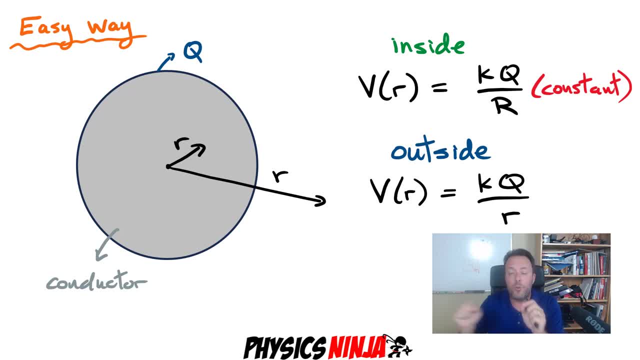 kq divided by the distance from the center to the point where I'm evaluating that electrical potential. The key point for this one is if you're on the inside of a shell or inside a conductor. the electrical potential is a constant value. okay, And the constant value? you calculate it by evaluating what is the potential at the 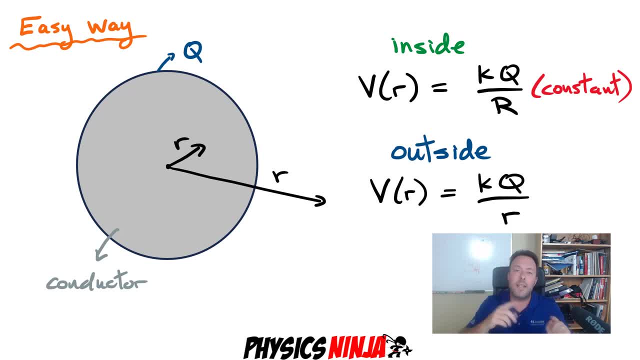 surface okay. If you use this result, it makes that other problem much, much easier to solve. We're going to show you both ways in this video. If you like the video, give it a thumbs up. If you don't like it, don't do anything. Alright, let's get started. Consider subscribing to my channel. 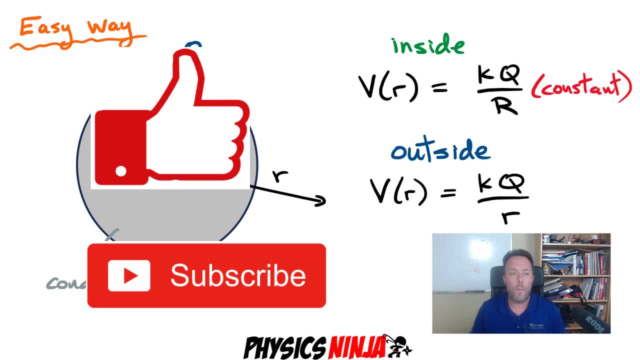 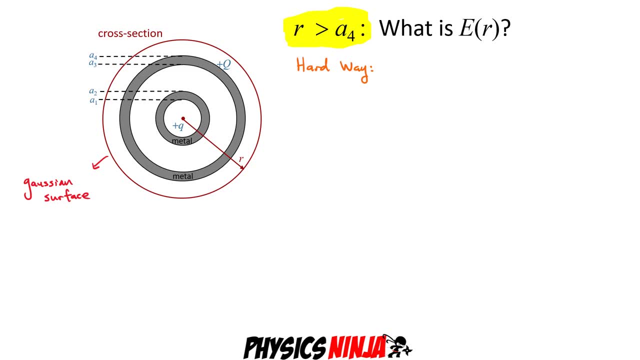 it's the best way to support what I do. Alright, let's go Alright. so the first thing we're going to do is consider the region where r is, the volume of the earth is bigger than a4. okay, so that means i'm outside of this entire object here. what i want to do is 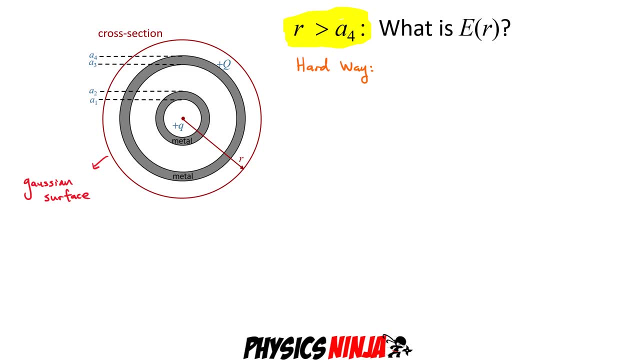 i need to evaluate the electric field out here in space. so i have a red gaussian surface here and i'm going to apply gauss's law to this. if you apply gauss's law to this problem here, the total charge enclosed now. well, think about it. you enclose this charge at the origin, little q. 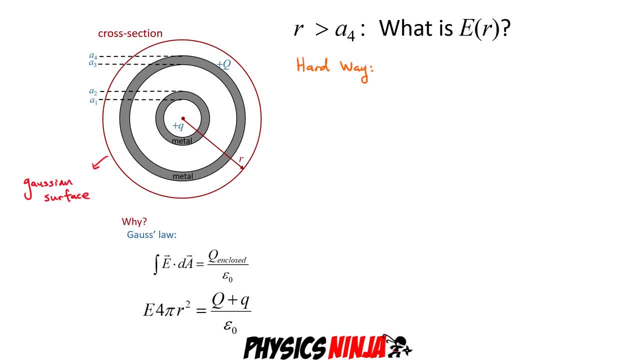 uh, this middle section has no net charge, so you don't have to worry about that. and now this outer shell has a positive charge, big q. so the total charge enclosed here is big q plus little q. all right, next thing you do, since this is a spherically symmetric object, 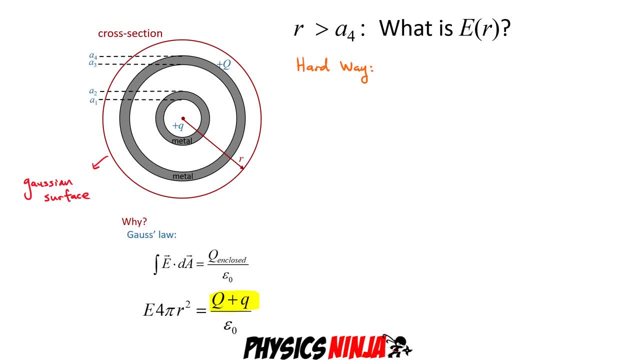 this side is standard for gauss's law, and now you can find the total field. now for the hard way. it says: well, you want to evaluate the potential difference between infinity? okay, we're going to choose infinity as our reference point here, because that sets this potential to zero. 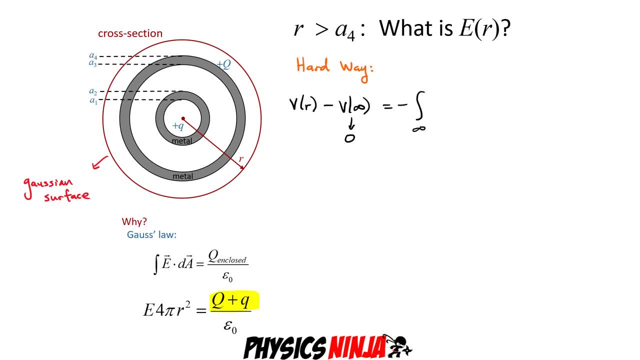 if i'm really really far away and i have to integrate from my starting point all the way to my final point, which is going to be somewhere on the sphere, what am i integrating? i'm integrating the field with the distance over here. that's the definition. so now what you have to do is 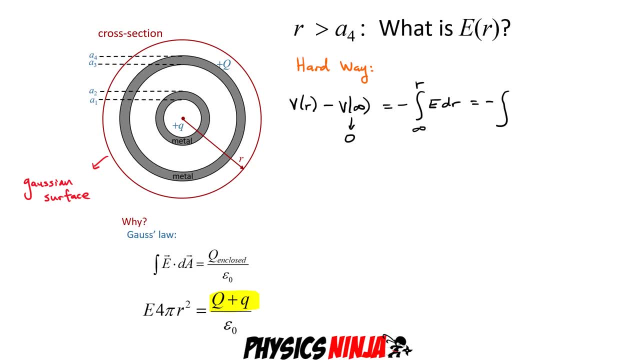 you need to simply substitute my definition for the field, so this becomes q plus little q divided by 4, pi, epsilon 0 and r squared and dr. now you can take a whole bunch of terms out of the integral and at the end you're left with this v of r. v of infinity goes to zero. and here i'm left. 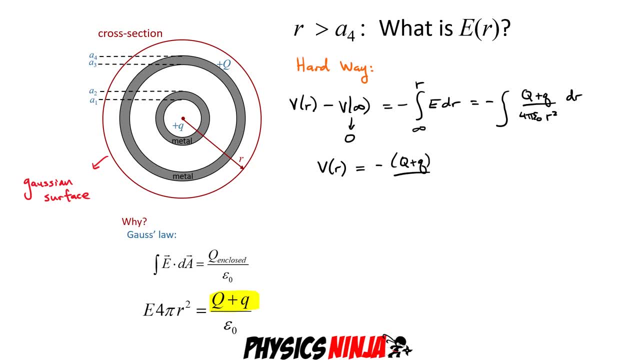 with minus. this is q plus little q divided by 4 pi epsilon zero, and i have to integrate from- sorry, from infinity all the way to little r. let's rewrite that and i'm integrating the function r squared. all right, we take this one step further: minus big q plus little q, four pi epsilon zero r. 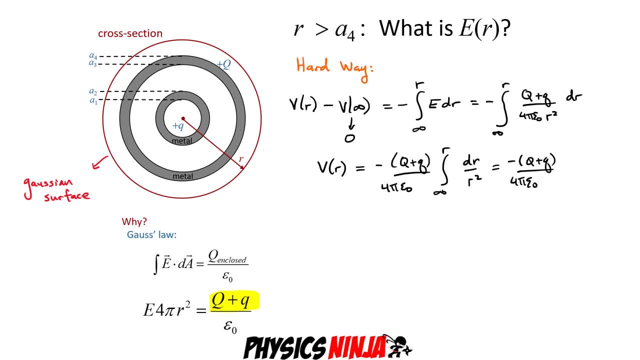 sorry, not r, let me skip that. i want to in evaluate this integral here. so the integral of 1 divided by r squared becomes minus 1 over r, evaluated between these limits, all right, and the last result you get, which is not that surprising, once you substitute those limits, those negative. 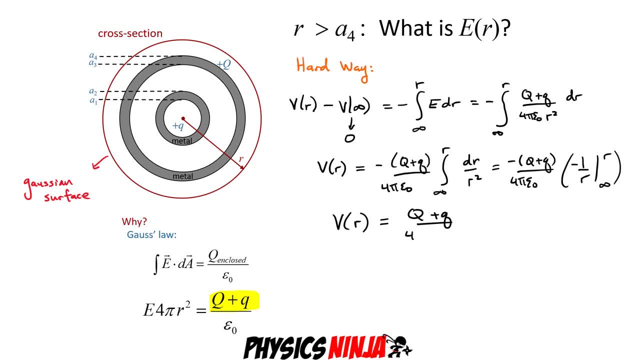 signs are going to cancel and you're going to be left with this and this here is the exact same result that you would get for a point charge. okay, the point charge right would have a magnitude of little q plus big q, and i'm a distance r away. so same result as a 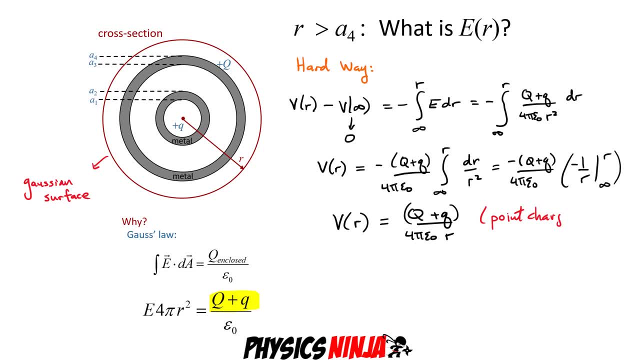 point charge. so guess what? i could have right away written that result, because if you are outside of a spherically symmetric object, right, it behaves exactly like a point charge, right? so the easy way, well, easy way, i would say, right away, i would simply write down my expression, the potential due. 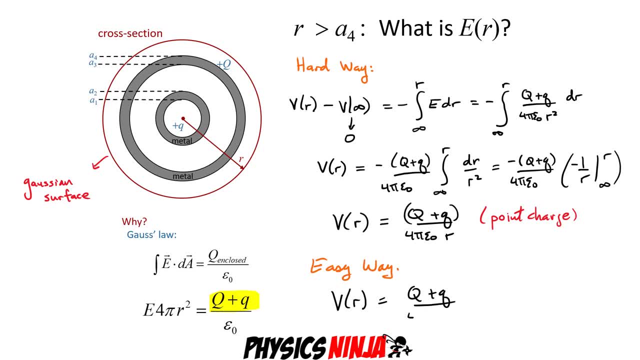 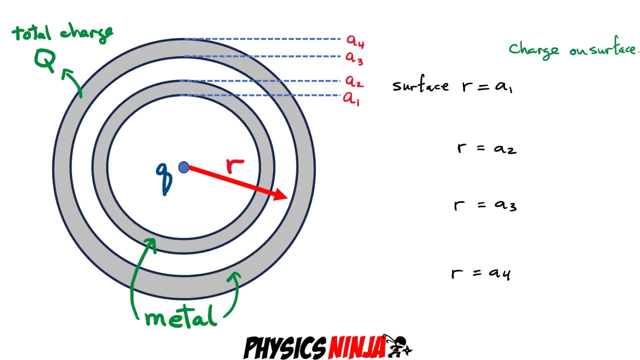 to a point. charge is q plus little q, divided by 4 pi, epsilon 0 over r. that's it. i would simply write it down, i'd be done. okay, you get the same result with the integral, as expected. all right, let's consider a different region now. all right, what we need to do now in order to calculate the electric 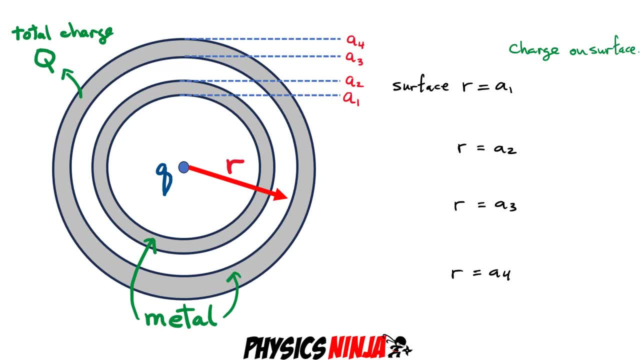 field. everywhere, we need to know what is the charge on each one of these surfaces. here right, there are many surfaces to consider. so we know we have a point charge at the center of both of these shells and we know the shells are made of metal. so if they're made of metal, you know that the 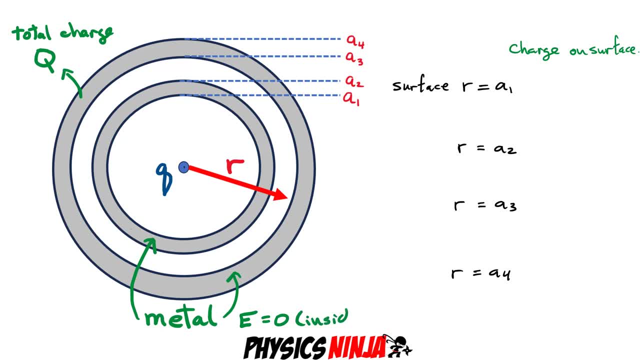 field has to be zero inside. okay, that is a requirement, and the only way you're going to have e equals to zero inside a conductor is if the total charge must be zero if i had a gaussian surface anywhere inside those conductors. so what does that mean? well, let's first consider this. 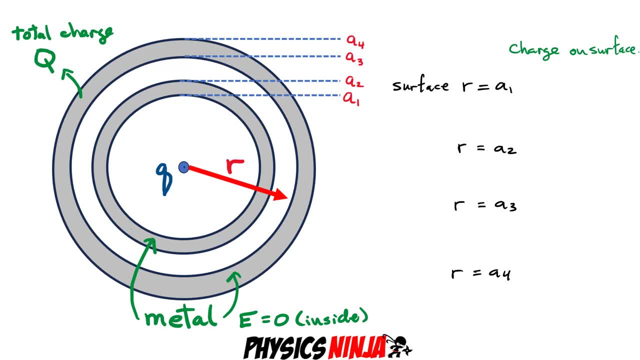 interior radius. here the smallest one, the inner surface of this first uh concentric shell. it has a radius a1. now if i'm enclosing a charge positive q, it means i better have a charge minus q equal and opposite to this one. so if i have a gaussian surface here, anywhere on the inside of 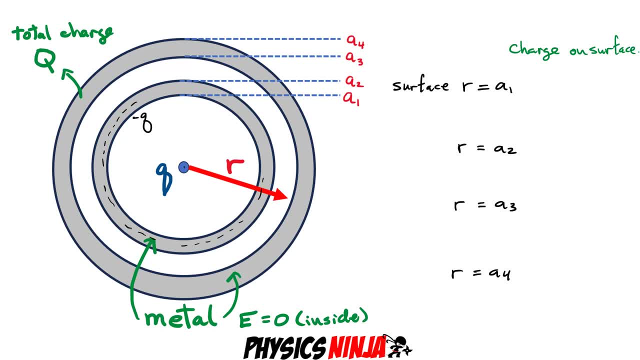 that conductor. i'm not going to draw the whole thing here, but let's just go quickly. you should have zero charge enclosed here inside this gaussian surface, and you're going to have that now as long as you have minus q that is on the inside wall. so let me go ahead and just right here, so on. 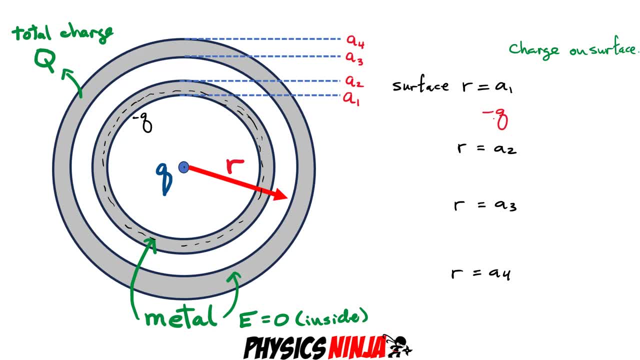 the outside wall, you have a charge of minus q. what about um on the outside wall? well, the outside wall, we know that this interior conducting shell is neutral. well, that means that on the outside wall, over here, you have to have plus q on this outside wall. so at a radius equal to a2. 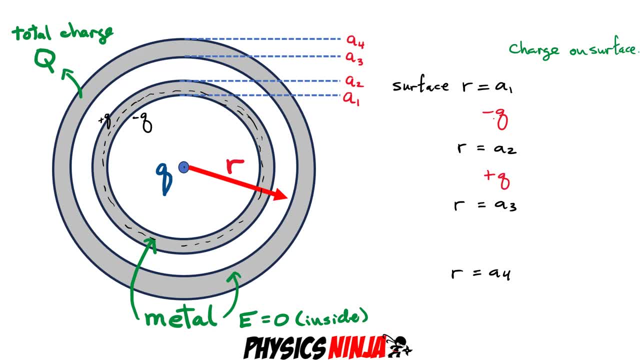 the total charge on that surface must be plus q and again it's going to be spread out uniformly across that surface. now we keep going on the inner wall of the outside shell, you're going to have to have a charge equal to minus q again minus q over here. 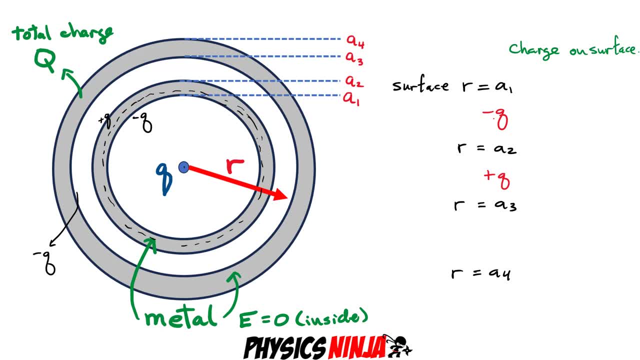 and on the outside. now you have to be careful, because this outside concentric metal shell right here has a total charge of q. so that means on the outside wall, guess what i'm going to have? i'm going to have a charge of plus q plus little q. right now you can. 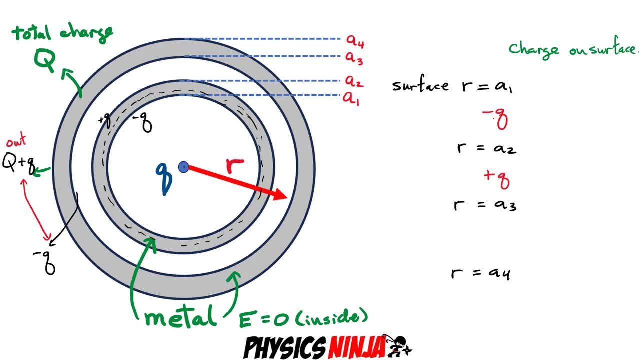 use these, both of these right, the wall on the outer and the wall on the inner. i'm still going to satisfy the requirement that the total charge is big q, so let's go ahead and finish this. so on this inner we have minus q and on the outer we have to have q plus little q, right away this. 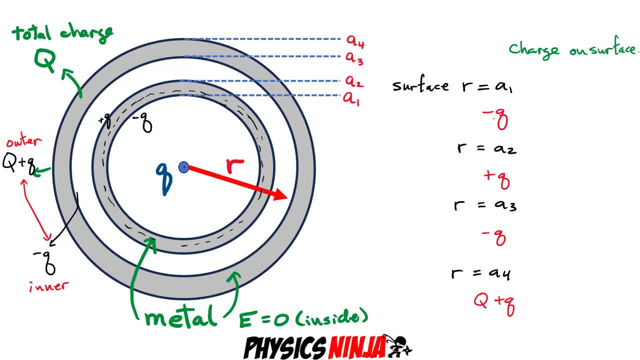 allows us to find the electric field everywhere, because you know how much charge is going to be enclosed now. because we know how much charges on each one of these surfaces find the potential very, very easily because we know how much charge there is on each one of those. 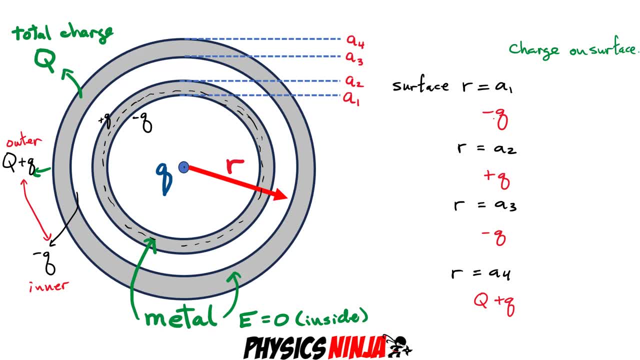 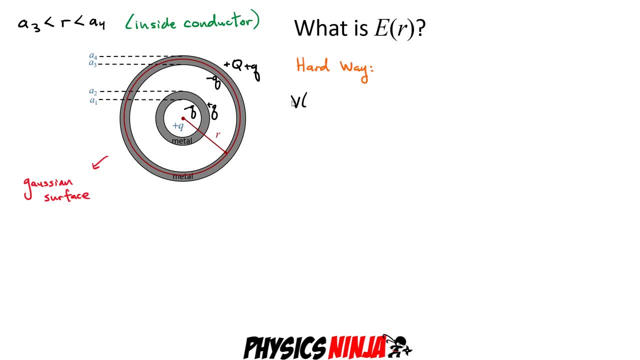 surfaces. so we can apply the hard way and the easy way right away. all right again, we apply our potential difference here. we consider the region now between inside this outer shell. okay, so we're integrating all the way from infinity, all the way to some position that's inside that region. 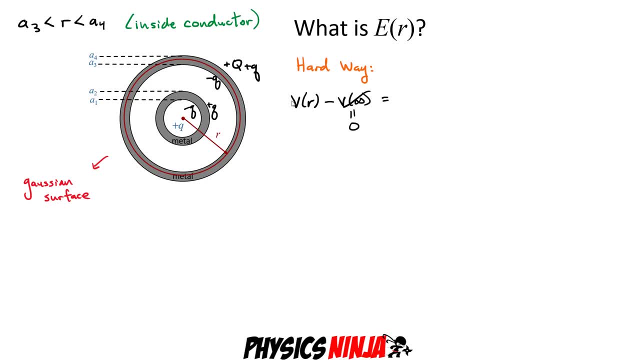 again, you don't have to worry about this. the reference is infinity. now we're integrating from minus infinity all the way to r of edr, and there's a minus sign in the front for that definition. now what you have to note is that the field varies. okay, the field is not constant. 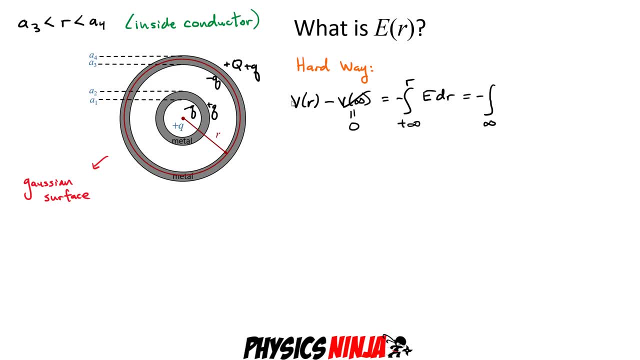 everywhere. so the field we know on the outside of that system. so what we have to do is you have to break this integral down. so first you integrate to this outer radius a4 and that's just the field from a point charge, like we did in the previous case. but we've changed this upper bound and now 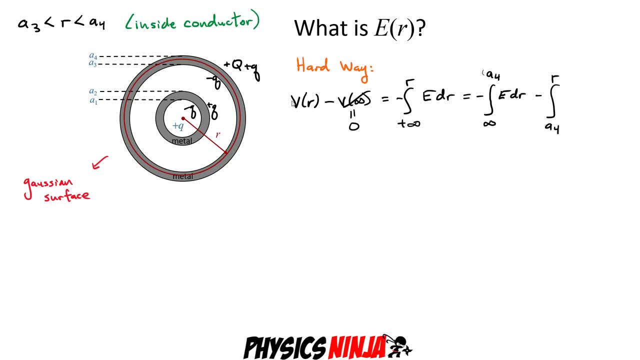 what we have to do is you have to integrate to this outer radius a4, and that's just the field from a4 all the way to my final destination, which is inside that conductor. except one important detail here, the field inside that region is zero right? so even if you integrate over dr. 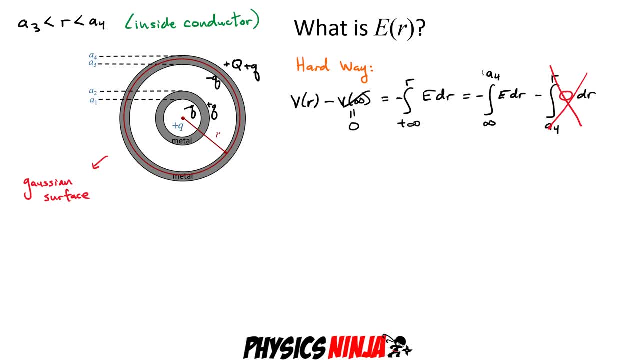 you are simply going to get zero for this term, so that makes the calculation simple. this is the exact same expression as what we had before, but our limits are different. so what you're going to find here is that, once you substitute both of those limits, you're going to get: 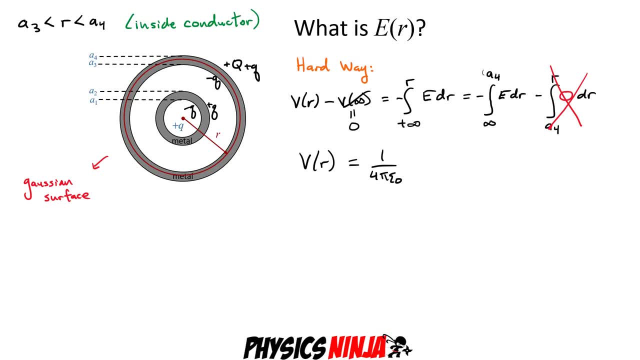 one over four pi epsilon zero. the total charge is q plus little q, um q plus little q. and now what else? the last thing is you have to evaluate it. within these limits you're going to get a4 over here. that's the hard way, right? the easy way is straightforward. the easy way, what you have to do, 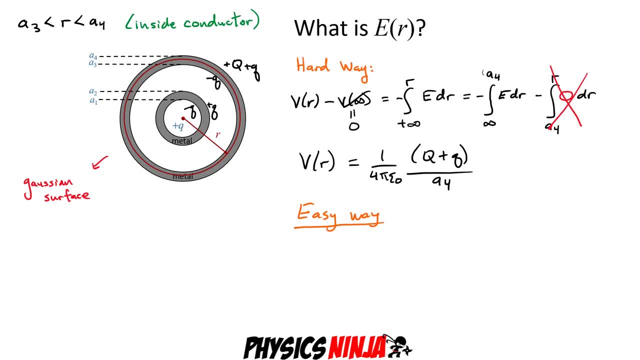 is simply consider the contribution from everything on the inside and everything on the outside. okay, everything on the inside is the positive charge q, and now we have all of these various charges. right, but if you're on the outside of these surfaces they behave just like point charges. and look at all the charge here inside. 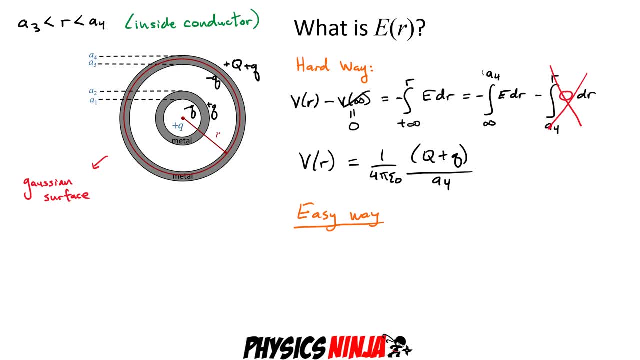 this, this surface, you basically have zero charge, so you don't have any contributions from any of these right, because we're outside of the surface and we're on the outside of the surface and we're outside of all of those regions and the total charge is zero. so they don't contribute anything. 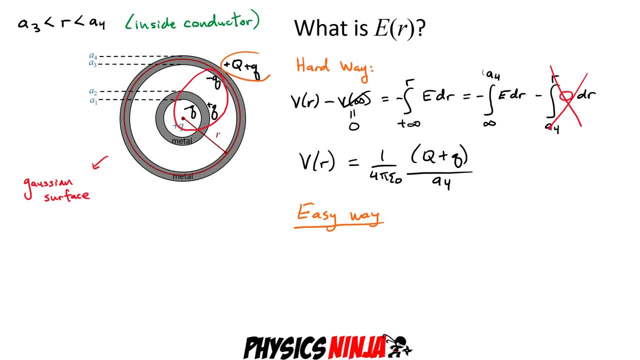 the only thing you have to consider is: what is the contribution from this? and now, since I'm on the inside again, I simply apply the rule on the inside. on the inside, the formula is simply the amount of charge on that surface, big Q plus little q, and divided by the radius of that spherical shell. 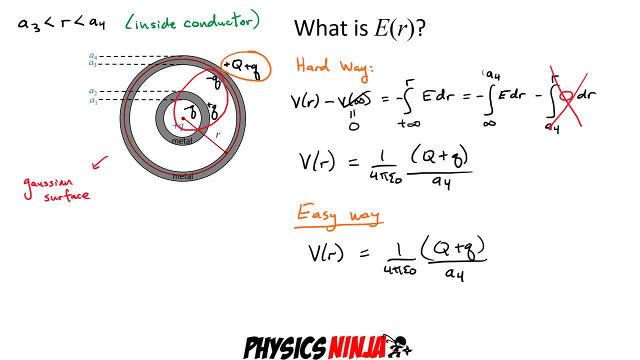 which in this case is a4. all right, so it's very, very important that we're going to be able to get easy to write down the result for this region. Now let's consider the region here shown in white between the both concentric shells. Alright now, if you. 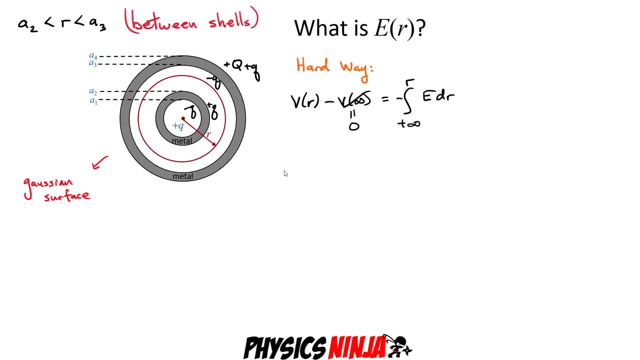 want to do this again now. we're evaluating the field in this region. here, What you have to do is you have to know the field everywhere in space, and we're going from infinity to R, So we know the field on the outside here, right this? 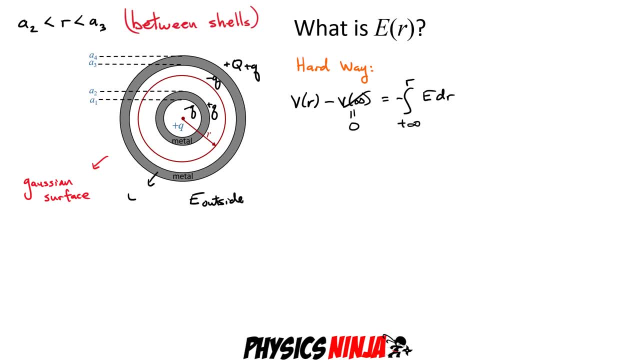 region we know. We know the field inside the metal is zero, so that's easy. But now you need to know the field here, anywhere inside this white region, here between the two shells. For that, if you apply a Gaussian surface like this, what you end up getting is that the field again. it only depends on how much charge. 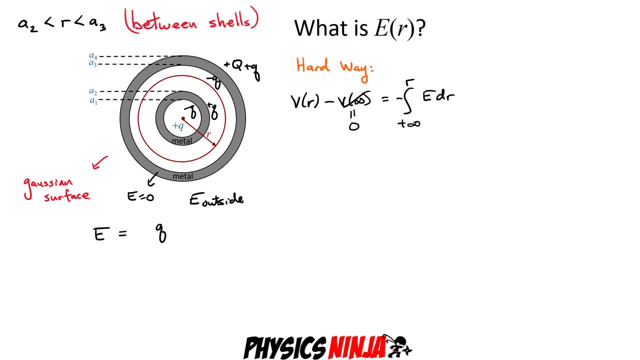 is inside And the total charge inside this Gaussian surface is little q only. So you get 4 pi, epsilon 0 R squared Alright. so this is the field between from A2 R all the way to A3.. So let's think about this integral now. 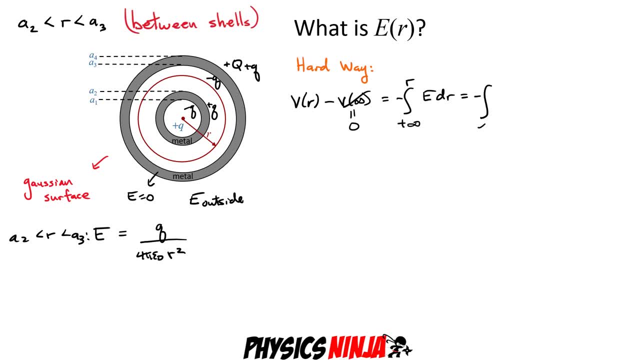 So let's think about this integral now. So let's think about this integral now. How would you do this? Well, again, I would break it down First. I have to integrate from infinity all the way to that outside region A4. And this is: 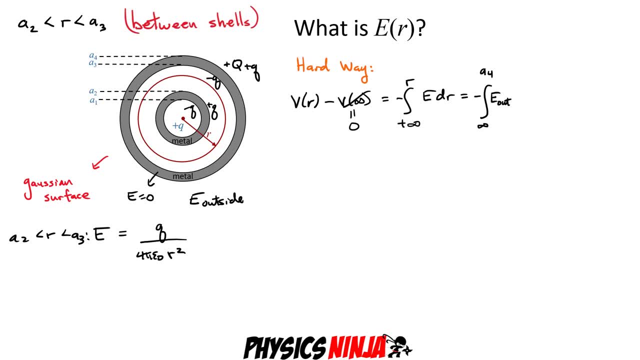 going to be the field on the outside. Just call it out- Okay, this expression over here that we used before. And then what? Well, now you have to integrate inside that shell. That's easy, because, guess what? the field is zero. There's not. 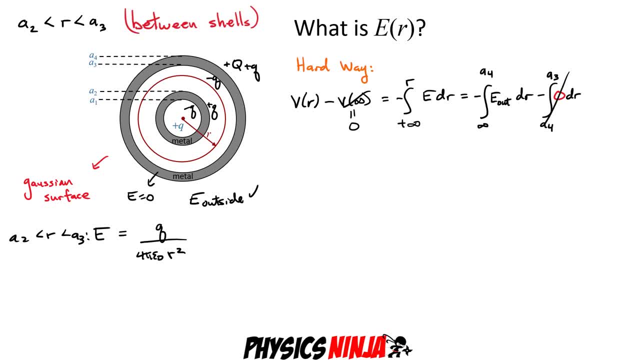 a lot of work to do there. Alright, so that's dr. So don't worry about this. And then the last little bit you can't forget: You have to integrate from A3 that inner radii of the outside shell, all the way to my final destination. And here we're just going to call that a kind of 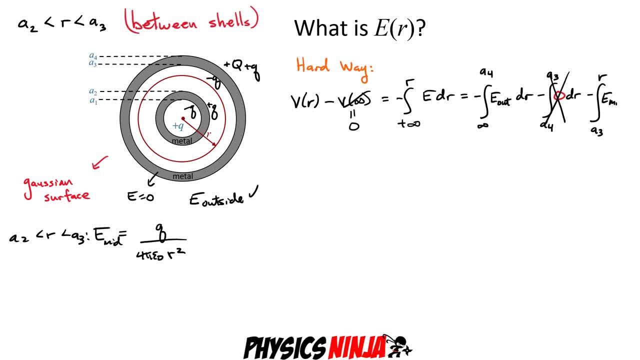 mid in that mid region. So this is the field I'm integrating over mid dr. Alright, so now we end up substituting our results inside and we simply have to evaluate these integrals. So this first term looks like what we just evaluated before. Alright, so that gave us K. This was q. 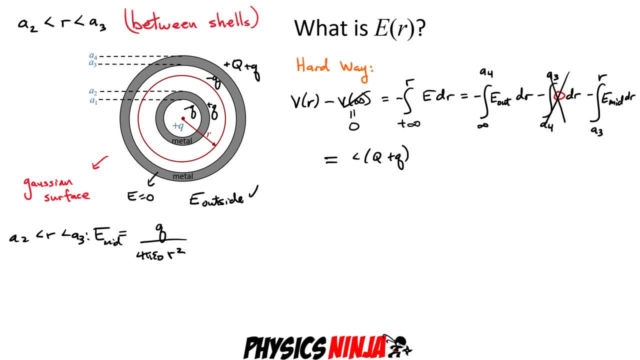 q plus little q, not k. sorry, I wrote it in terms of 4 pi epsilon zero, trying to skip a step here. 4 pi epsilon zero multiplied by, divided by a4. over here, the second integral is zero. and now 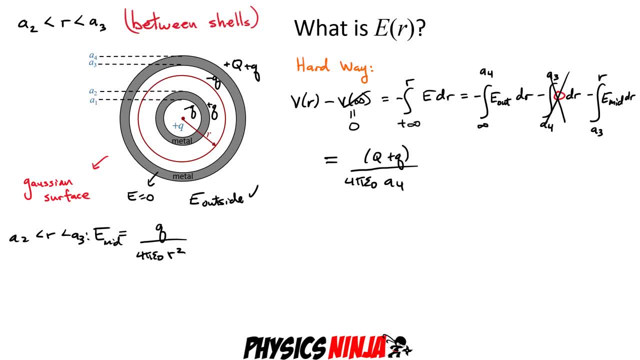 this last one, you have to be a little bit careful, okay. so what you're going to get is plus a little q, 4, pi, epsilon zero. this gives me a 1 over r, and I'm evaluating this between a3 and r. 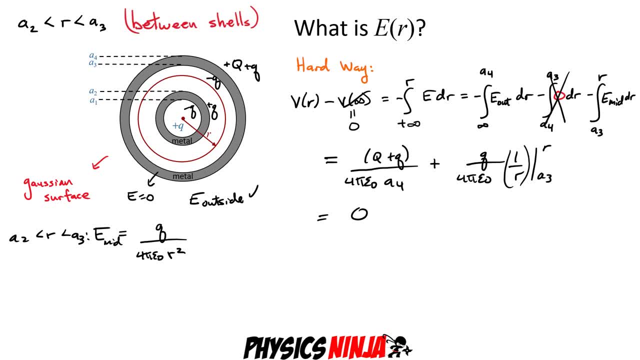 okay, this function. so you have to evaluate this integral. now this one looks pretty complicated. you get various terms over here: a4, and now, once you substitute these limits, you get q, 4, pi, epsilon zero, and this becomes 1 over r minus 1 over a3,. all right, and this is. 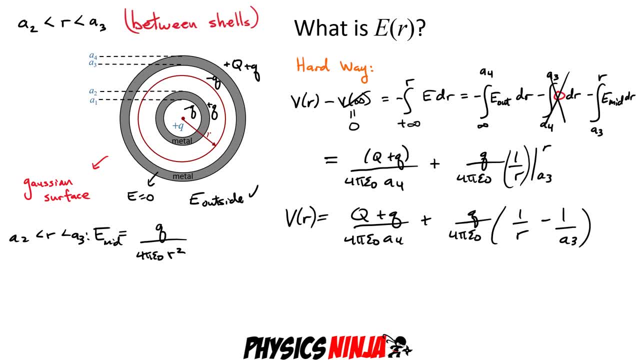 the potential anywhere inside that region. you notice, it depends on the distance. now, it also depends on these other guys, right, which ended up being the contributions from the outside and the inside shell. so now let's think about how we would do this. the easy way: 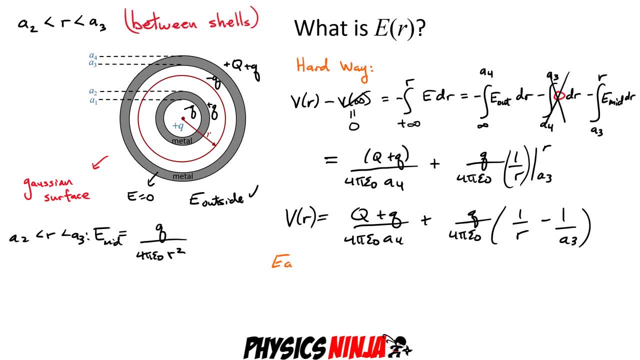 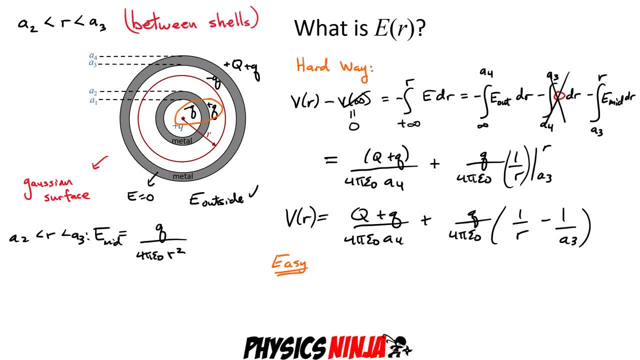 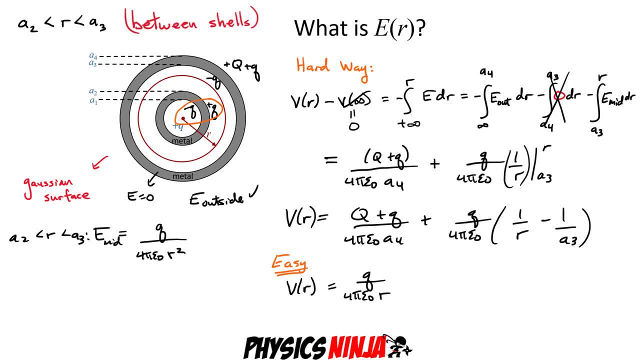 other terms that contribute to the potential right. There are both of these surfaces. This surface here has a charge, big Q plus little q, and this inside surface also contributes to the potential. What do they contribute? They contribute constant terms. So this is what it looks like, You. 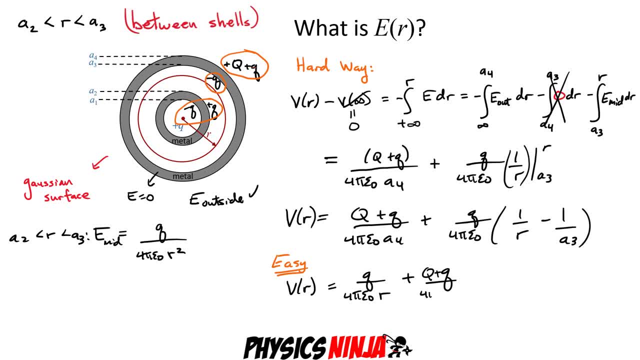 get big Q plus little q, 4 pi epsilon 0,, and that is a radius A4 away. And now you also get this charge minus Q over here. The minus Q is minus Q, Its contribution is 4 pi epsilon 0, and its radius 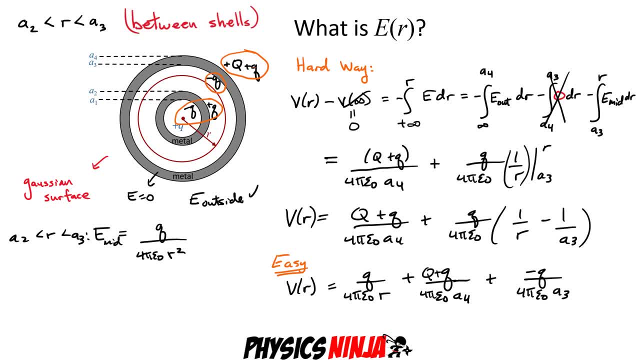 is A3.. Okay, you could see, right now you can kind of get rid of this. just clean this up a little bit. Maybe bring that negative sign And, lo and behold, you will get the same result as the harder way. However, for me it's much more straightforward just to write down. 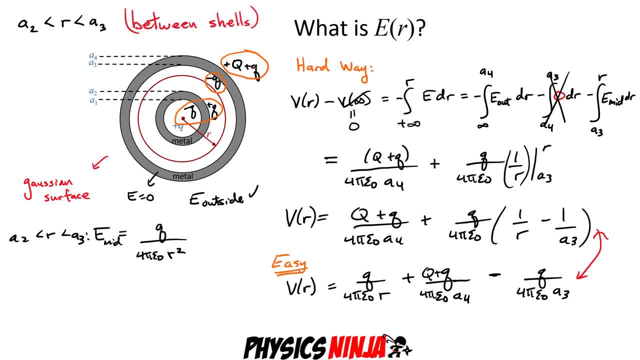 these three contributing factors than to evaluate all these integrals. But you can see, we all have the same terms and they all have the same sign, All right. so using this analysis, we can evaluate it anywhere in this region. So I'm just going to do one more. I think you should at this point. 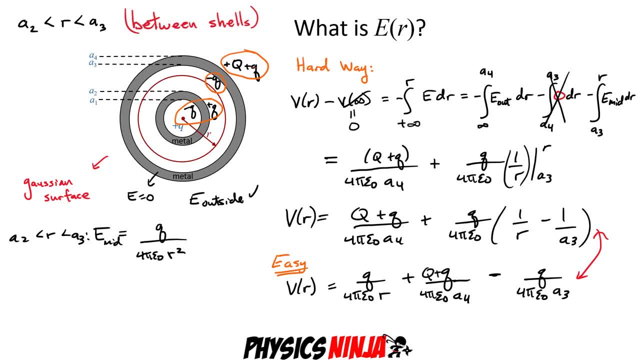 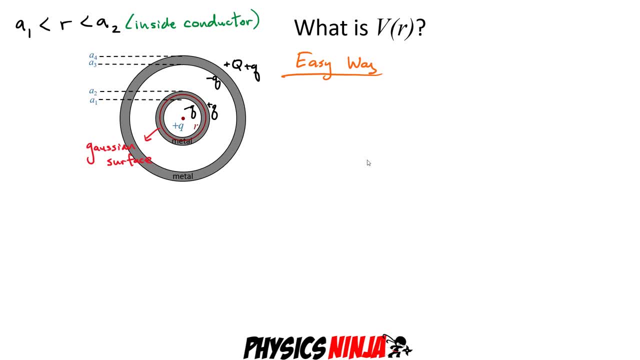 understand the technique, So let's just pick one. One more region to finish off the problem. All right, what I'm going to do now is consider the region here in this, inside the conductor over here, What we know is that the field inside that 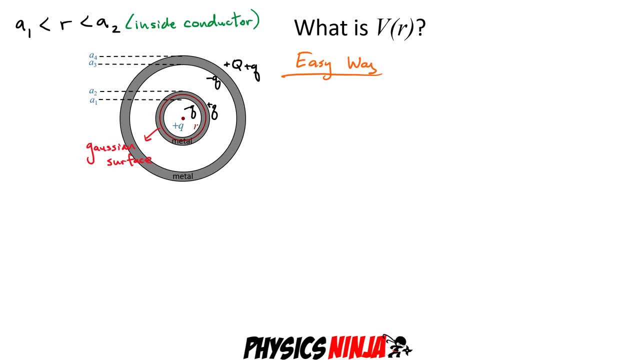 conductor is zero, right? Therefore, the potential actually has to be a constant inside this shell, right? So again, this is the region I'm considering between A1 and A2.. That's the inner and outer radius of this inner shell, And I'm going to get lazy. 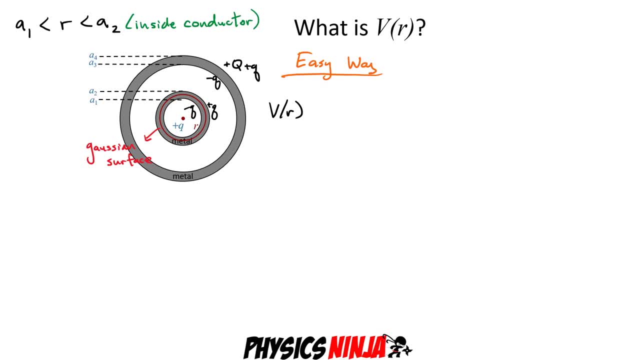 We're just going to write down the result. So think about it For anything on the inside. look what we have. There is no net charge here on the inside, because I have minus Q on this inside wall and I have a plus Q right here at the origin, So those two don't contribute. 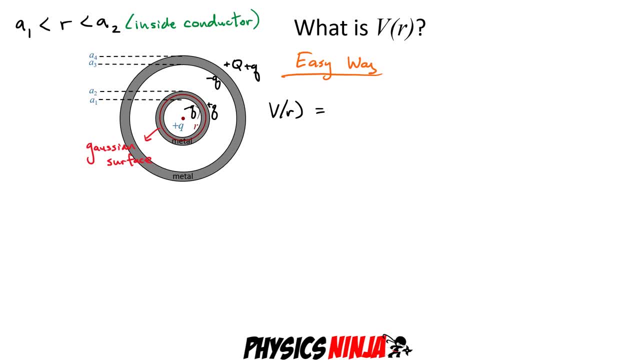 anything to the overall potential. What we do have is we have three surfaces here that contribute constant terms to the potential, So the total potential is going to be a constant. All right, I'm going to factor out the 1 over 4 pi, epsilon zero, because that is common. 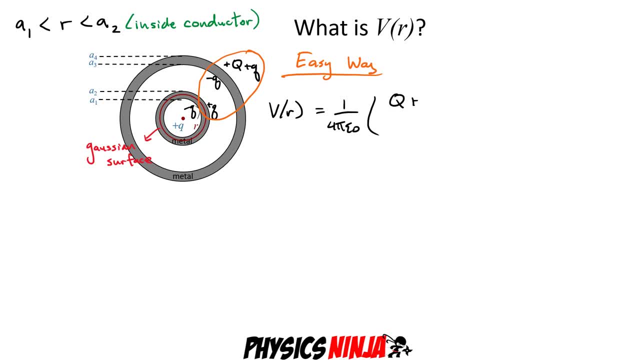 for all the terms, and this is what it looks like. So, for that outer shell, this is the contribution. It's this, okay, It's the charge divided by the radius of that shell. For this inside wall here, what does that contribute? That is Q divided by A3.. And now, what else do we have? 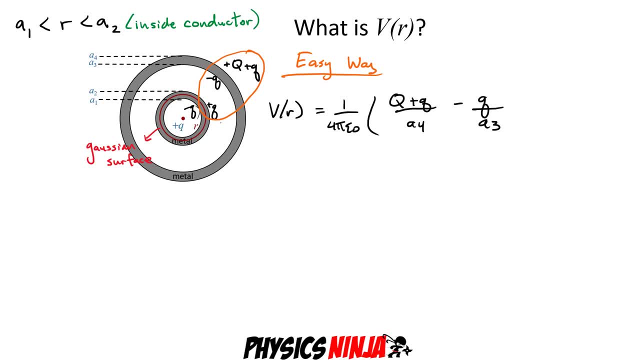 Now we have this new term because we have charge on the outside surface of this interior shell. Well, that contributes a term of Q divided by A2, okay, Notice that this electrical potential is a constant value. okay, Everywhere inside that region. That's because metals are equipotential. 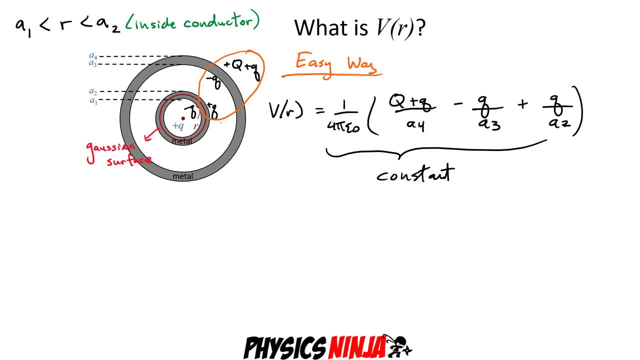 surfaces okay. They have to have a constant potential. So pretty straightforward to evaluate that guy, All right. so the last region I need to consider is all the way on the inside- both of them, And the only charge that's enclosed is this positive charge. right, if you consider a? 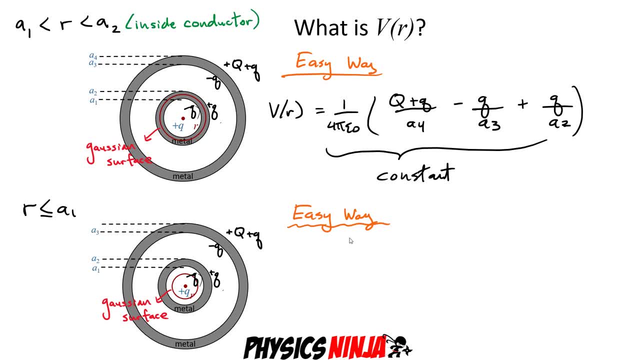 Gaussian surface. So the electric field is just plus Q divided by 4, pi, epsilon zero divided by R squared. But the electrical potential then has five contributing terms. right, You're going to have the contribution from the charge right at the center. Guess what That simply behaves like. 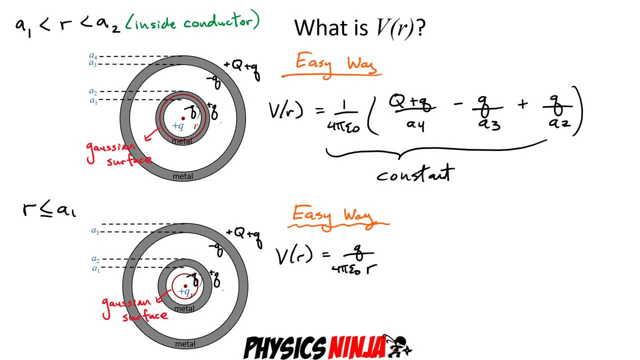 the potential of a point charge Q over R. Now we have the potential of a point charge and we have the potential of a point charge Q over R. Now we have the potential of a point charge and we have the four surfaces that we have to consider. All right, so we have first the surface at a radius A1.. 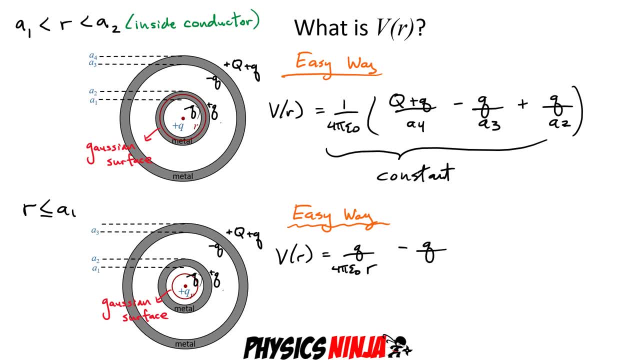 That contributes a term of again. actually, what I should have done here is I'm going to factor out a 4 pi epsilon zero, because it's going to appear in all of the terms. So, if you bear with me here, we're going to do some magic here. Let's move this down, Let's move this over, so I can bring. 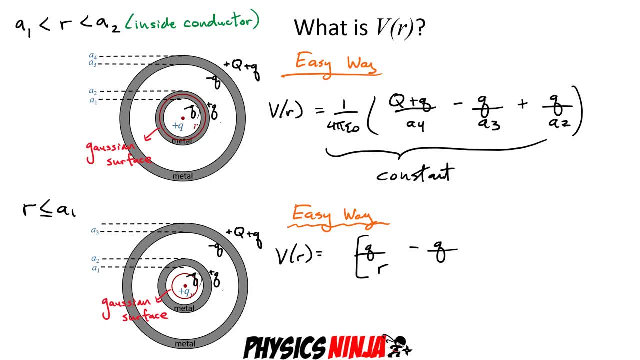 over the 4 pi epsilon zero. Okay, This is going to make the expression look cleaner. All right, so the contribution from this inside wall right here: it has a charge minus Q, so it contributes a constant term equal to Q divided by. 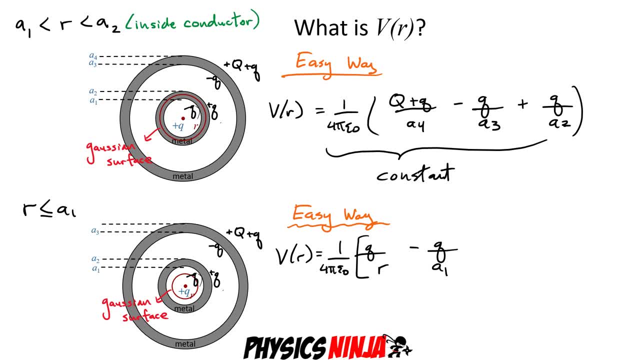 A1. The outer surface contributes to the electrical potential. a term of its charge divided by the radius here is A2, right, This here becomes the same terms as up above. Then you get minus Q over A3, and then you get minus Q over A3. And then you get minus Q over A3. And then you get minus Q over A3. 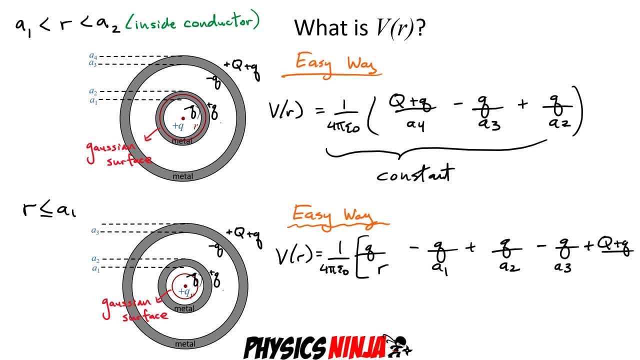 Plus Q plus little q, the charge on the outside divided by A4.. Okay, Complicated looking expression. It depends on the distance, right? Okay, Similar to a point charge for this one, but you have all of these extra terms here that contribute a constant term to the electrical potential. 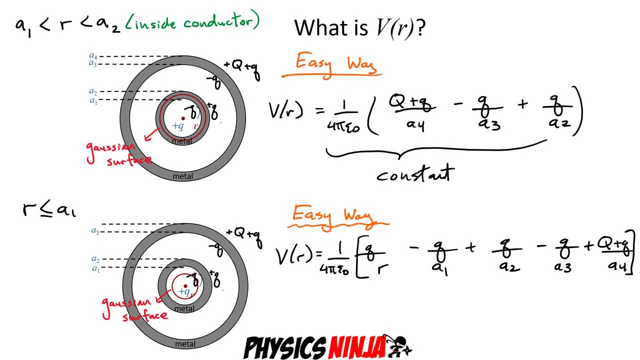 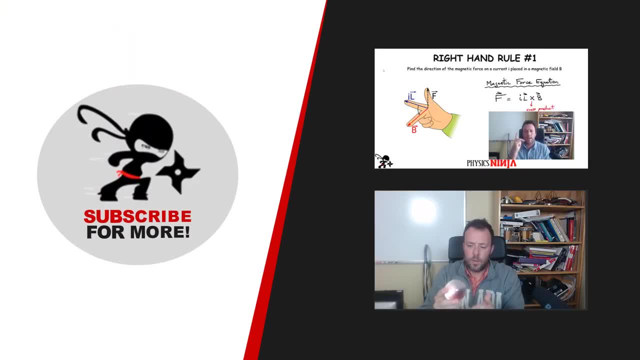 All right, folks, that's it for me. Hopefully, you got something useful out of this video. Thanks for watching. I'll see you next time. Thanks for watching. I'll see you next time.